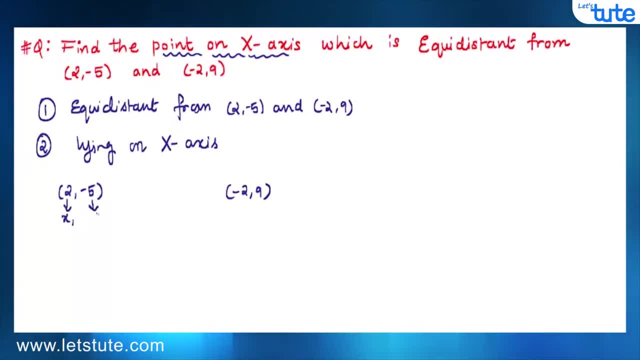 point. let us say the x coordinate of the first point is x one, y coordinate of first point is y one. x coordinate of second point is x two and y coordinate of second point is y two. and we need to find the third point which we don't know, the coordinates of the third point. so let us say the coordinates. 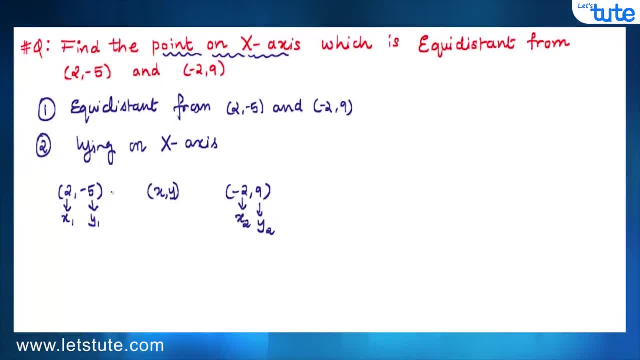 are x and y. only thing we need we know is there they are. the two points are at equal distance from this point. okay, so that is from the first condition. now the second condition says the point is lying on x axis. what do you mean by that? let's understand that from. 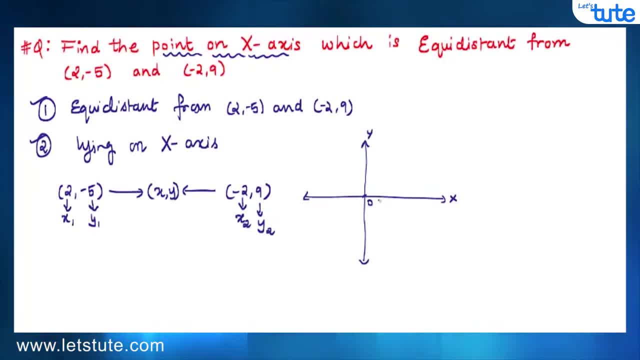 this coordinate axis, this is x axis and this is y axis. now we know that the points on x axis we generally write in this way: one, two, three, four. what do we understand by that? this one is basically one comma zero. this two is basically two comma zero. this three is three comma zero. 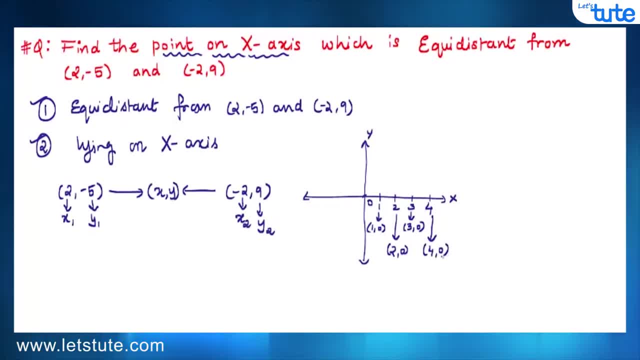 and this four is four comma zero. So what do we get from this? whenever a point is on x axis, its y coordinates- look at them- its y coordinates will be zero. similarly about this point: since this point is lying on x axis, we will have y coordinate as zero. so this point finally looks like this: x comma. 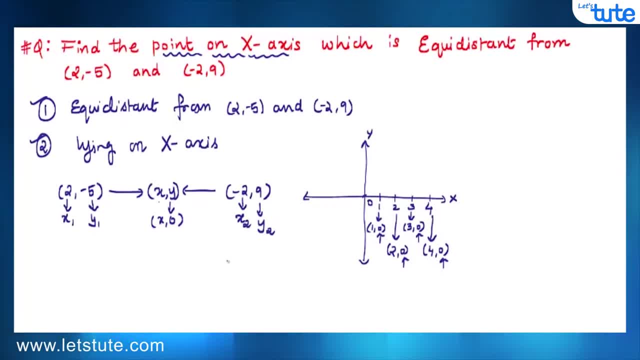 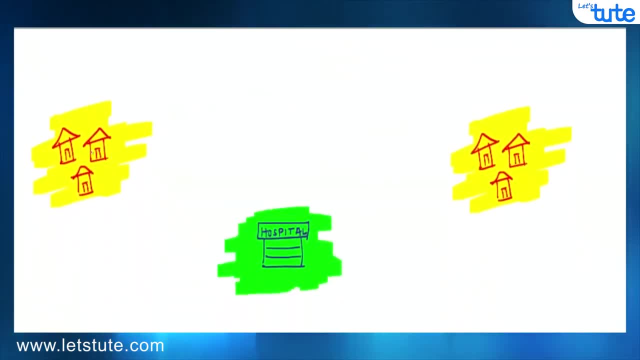 zero, got it fantastic. let's understand this with a real life example. let us say: let's go down. Let us say there is a situation: we have village, two villages, this is village one and this is village two. so for time being, let us say v one for village one and v two for village. 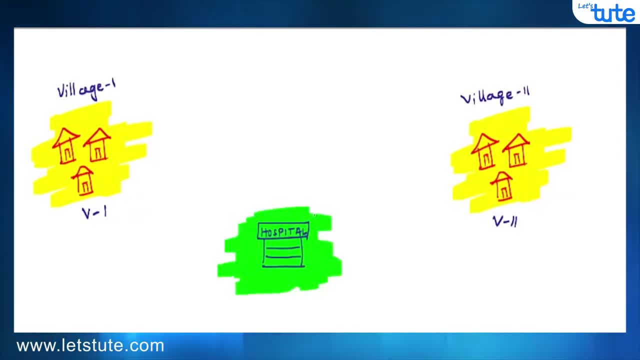 two and a government wants to build a hospital between village one and village two. but the condition is distance from village one to the hospital To the hospital should be equals to distance from village two to the hospital. that means suppose d one is the distance from village one and hospital, that is v one and hospital. 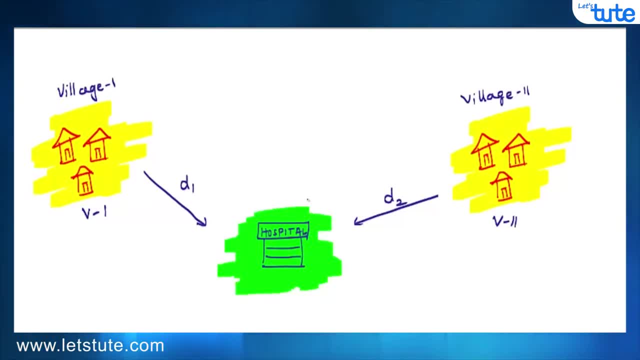 and let us say d two be the distance from v two to hospital, then d one has to be equals to d two. okay, so let's understand with this question. suppose two comma five, two comma minus five is the coordinate for village one And coordinates for village two. say minus two comma nine, then we need to find xy for 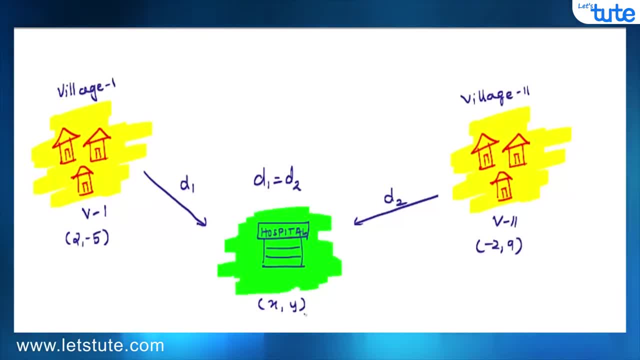 the hospital. that means the coordinates of the hospital and the condition is the hospital. that means the third point is on x axis, which we already know from the question, and we already said that when point is on x axis, the y coordinates become zero. so now the coordinates of the 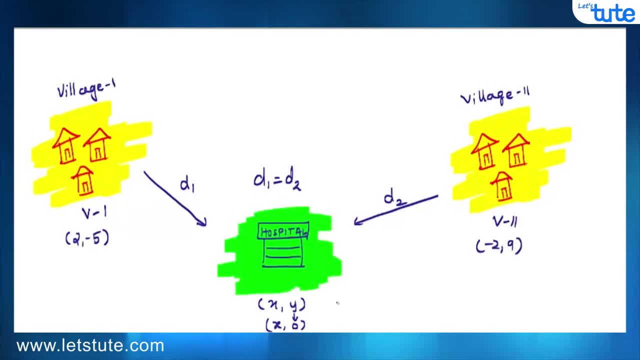 hospital is x comma zero. Let's work out this. What will happen? We know the distance formula. Suppose we have two points- x1, y1 and x2, y2- and we want to find distance between them. Suppose that distance is d, then d will be equals to square root of x1 minus x2, the whole square plus y1 minus. 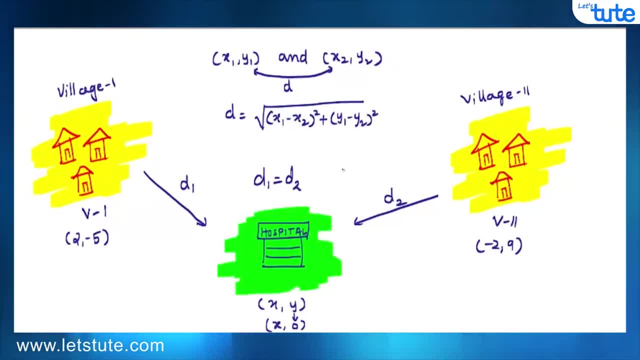 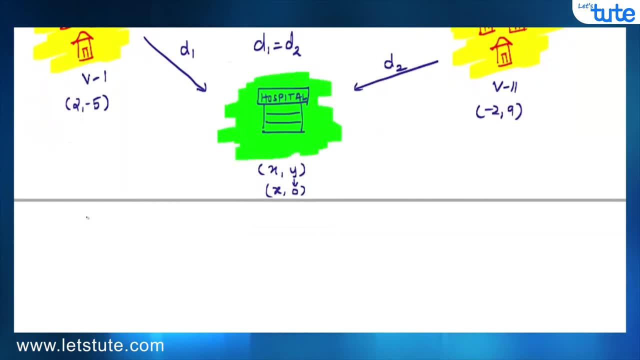 y2, the whole square. This is what we learnt. Let's apply that. Let's go down a bit. Let's first find distance 1, that is, distance between village 1 and the hospital. Okay, So for that we will use the coordinates of village 1 and the coordinates of the hospital. 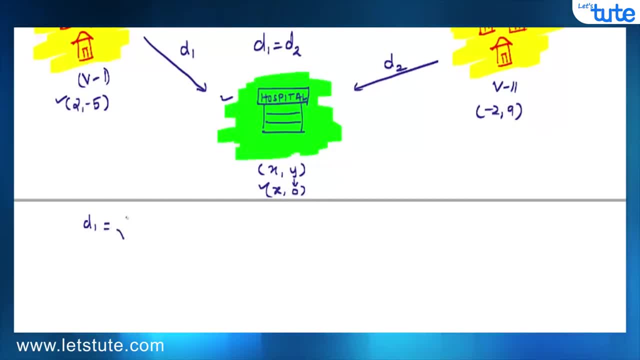 So using the formula which says: square root of x1 minus x2, the whole square, plus y1 minus y2, the whole square. So for this reason, let us take this two as x1 minus 5, as y1 plus x2, and here let us take this x, this x as x2 and this 0 as y2.. Okay, Fine, then let's. 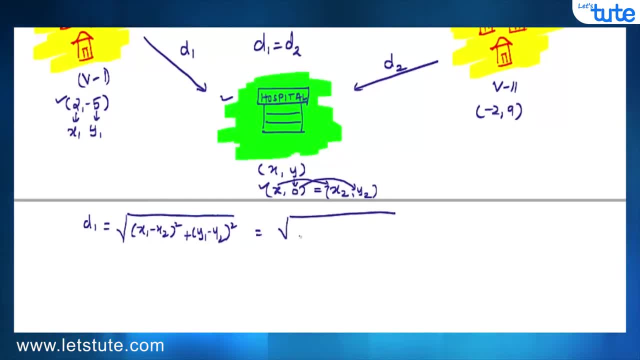 apply this, What will happen here? Let us see: x1 is 2 and x2 is x- whole square plus y1 is minus 5 and y2 is 0- whole square, Correct. So, after solving this, what we will get? Let 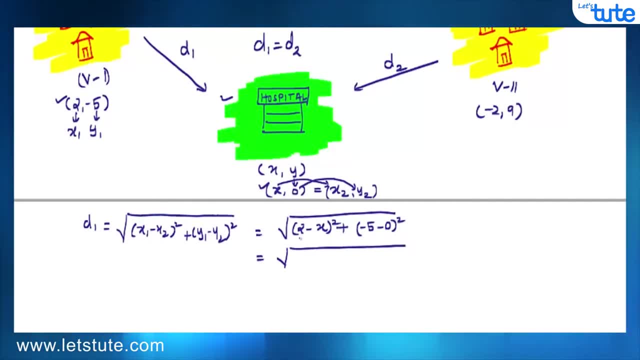 us see We will get. we have to apply a minus b whole square formula. We all know that what is a minus b whole square? a squared minus 2ab plus b squared. So we have 2 in place of x and we have x in place of b, Correct? So after applying this, we will get a minus. 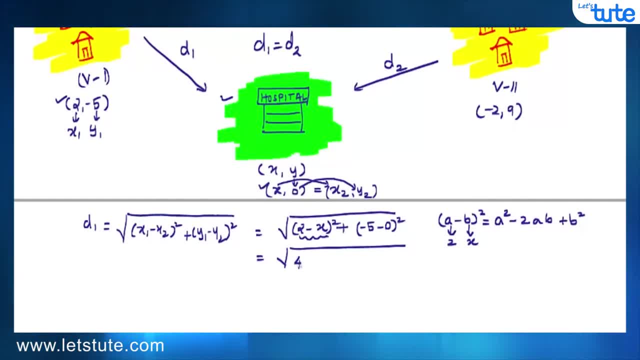 b whole square. So after applying that, what we will get? We will get 2 squared, that is 4 minus 2ab, that is 4x plus b. squared, that is x squared. Okay, And here minus 5 minus 0 will be minus 5.. Correct, I will write over here: minus 5 minus 0 will be minus 5.. So taking: 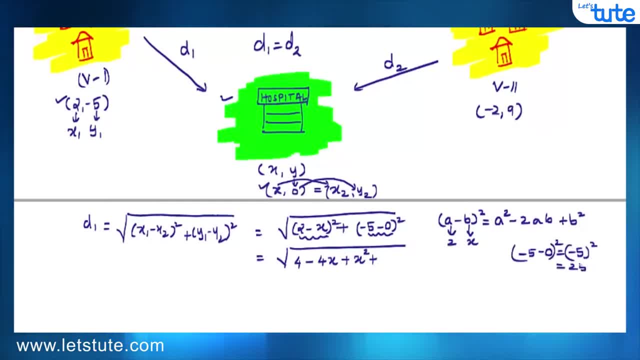 the square. what we will get? We will get. we should get 25.. So I will apply here 25.. Fine, After simplifying, what we will get, We will get x squared minus 4x plus 29.. Great. Similarly, let's find d2.. Let's go down. 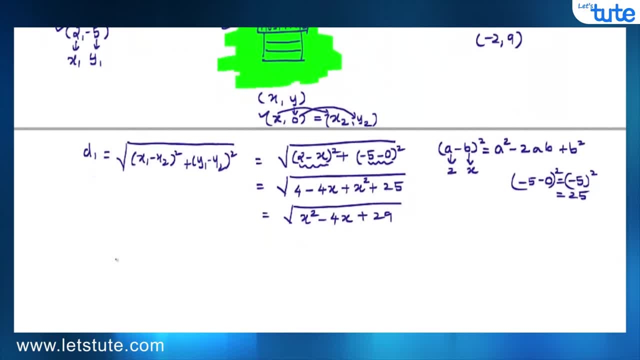 a bit D2.. Similar formula we will apply: Okay, x1 minus x2, the whole squared, plus y1 minus y2, the whole squared. Okay, And here, for this reason, let us take this as x1 and this as y1, and we already have x2- y2.. So let us apply. 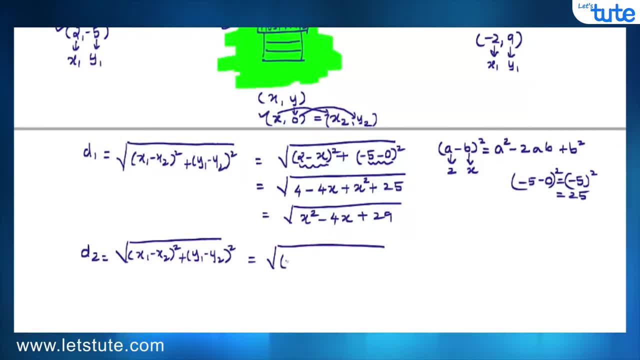 that what we will get here. We will get x1, that is minus 2. minus x2, that is x whole squared plus y2.. Okay, Okay, Y1, that is 9.. Correct, You can see here, Minus y2, that is 0.. Fine, So let's simplify. 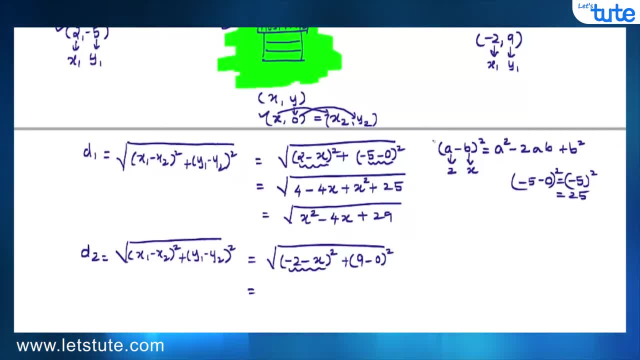 this: We are going to apply a minus b, whole squared formula, as we did over here. So what we will get? Let us see that We will get a squared that is minus 2 because we have. in this case, if we go a, we have minus 2.. Okay, So we will get a squared that is minus 2 because 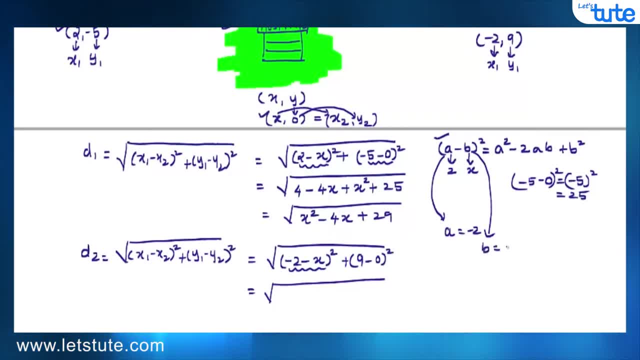 we have x Correct, So we will apply the formula. We will get a squared, that is minus 2, squared minus 2ab, So 2ab plus b squared, and here 9 minus 0.. What will be 9 minus 0?, That is. 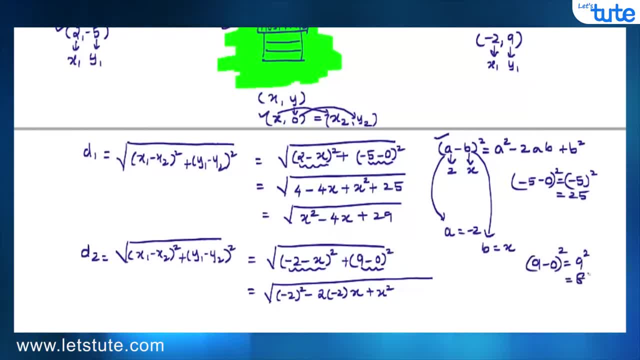 9 and squaring them, we will get 81.. Okay, Fine, So this will be 81.. So let us simplify this and see what we are getting. We will get: minus 2 squared is 4, and this is plus 4x plus x, squared plus 81.. So, after simplifying, 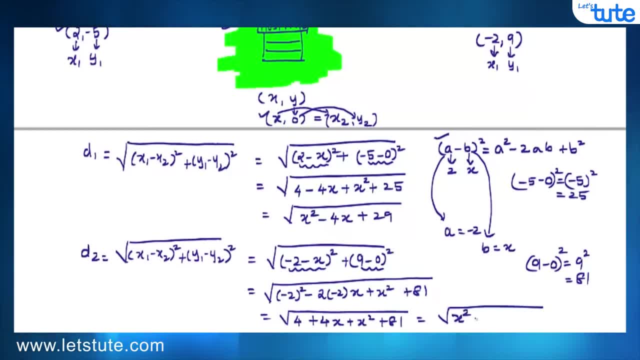 further what we will get. We will get x squared plus 4x plus 81.. Sorry, 85, because we have to add this 4.. Fine, We got d1.. This is our d1.. Let me put it in red box: This is our d1.. Okay, This. 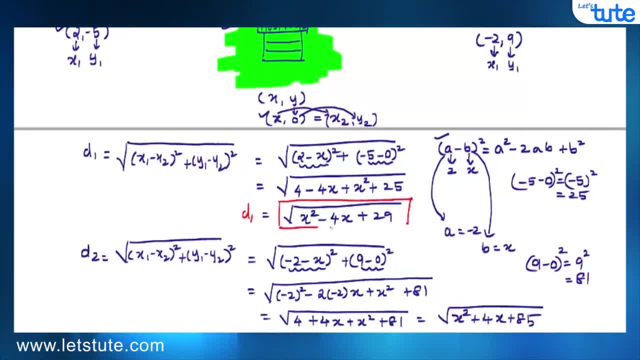 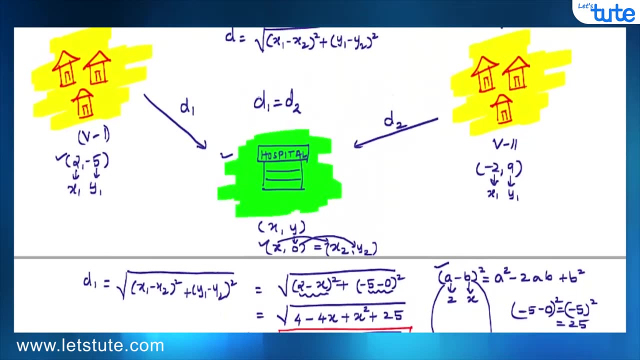 is our d1.. Fine, And this is our d2.. Let me put this as well in a box. Okay, This is our d2.. Now, according to the condition: What is the condition over here? We have to see this. 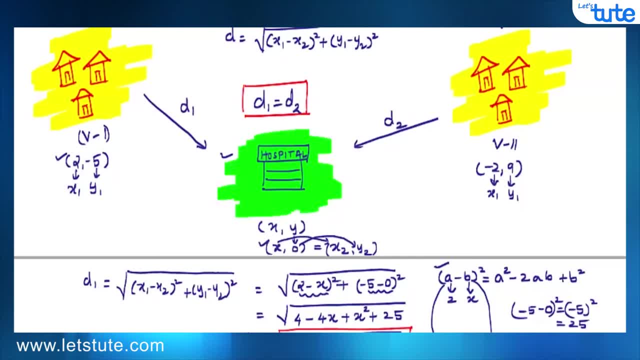 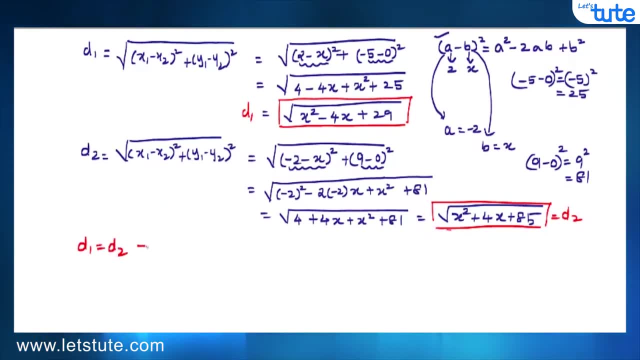 The condition is: d1 has to be equals to d2.. Fine, let us equate them. Okay, When we equate them, d1 equals to d2, what we are getting We will get this, that is, d1 is x squared minus.